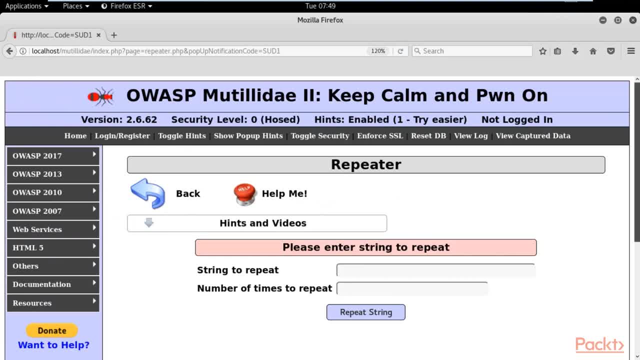 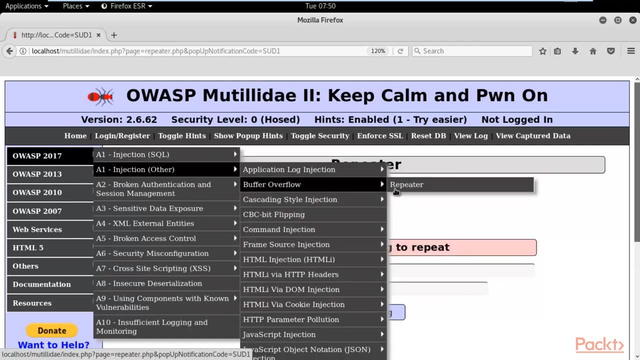 So here this is OS Matilide, and we need to perform buffer overflow attack in the web application. So to do that, let me find out the buffer overflow. So select OS 2017, select injection- other attacks- and then you will find buffer overflow and click on repeater. 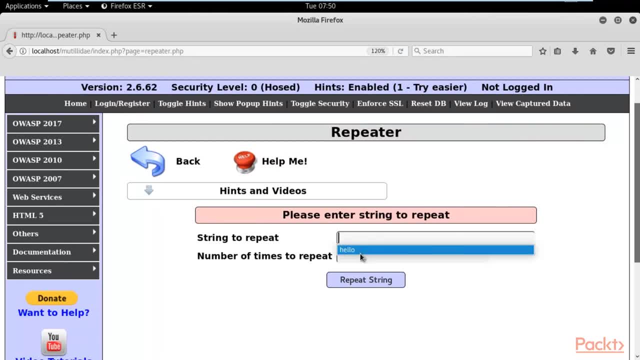 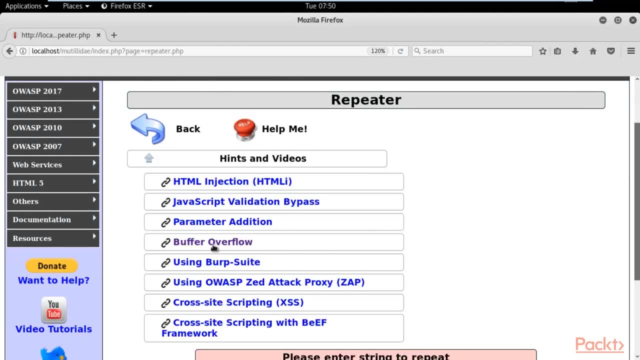 So here it is Right. repeater. please enter string to repeat and number of times repeat. Before that I need to check the theory behind it. Let me click on hints and we will see how it works. So this is buffer overflow, right? 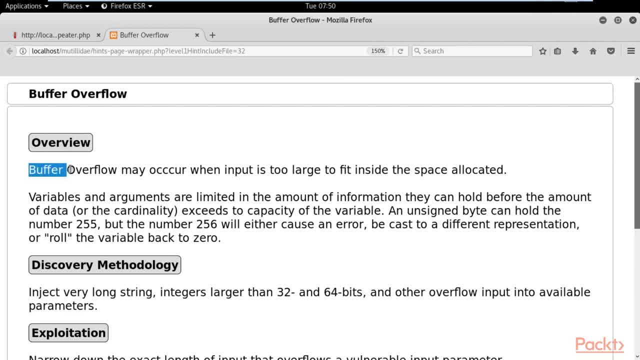 What is buffer overflow? As I already told you, but let's repeat it, Buffer overflow may occur when input is too large to fit inside the space allocated. I already told you that space is less and you are putting more data inside it. This is called buffer overflow. 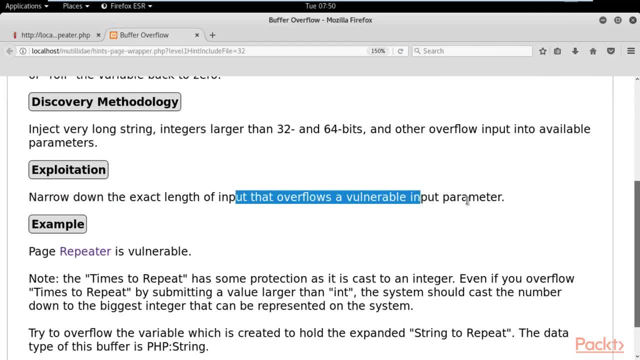 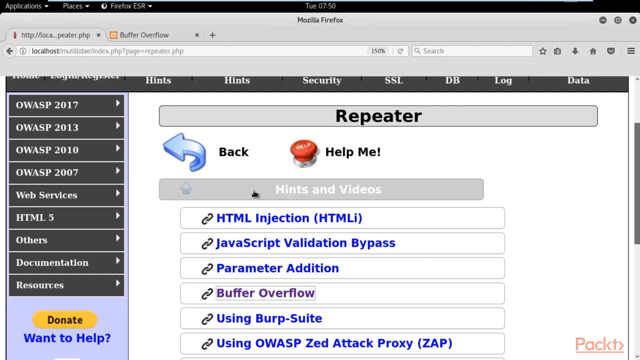 So narrow down the exact length of input that overflows the vulnerable input parameter. This is the exploitation right And this is example. Page repeater is vulnerable Right. This is the page repeater which is vulnerable And the times to repeat has some production and it is cast to an integer. 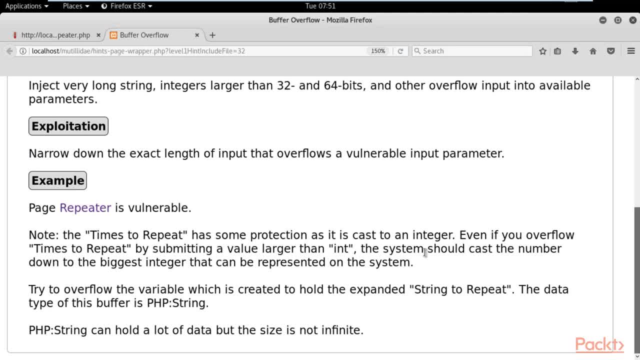 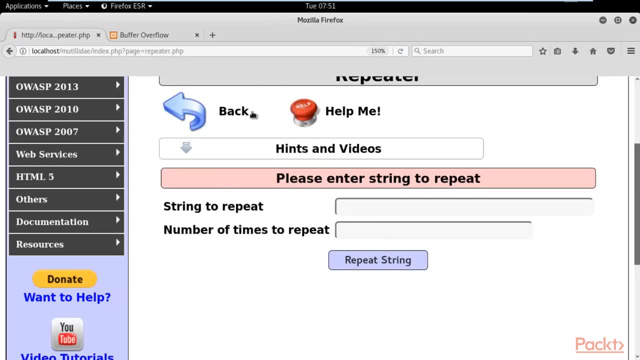 Even if you overflow times to repeat by submitting a value larger than int, the system should cast a number. The thing is quite simple. You can insert any amount of data inside this web page, right? And this should not happen in actual web application. 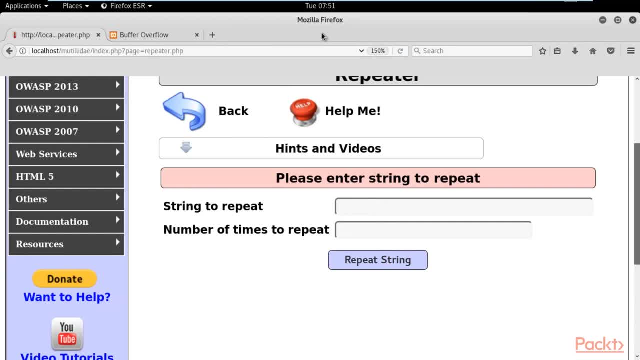 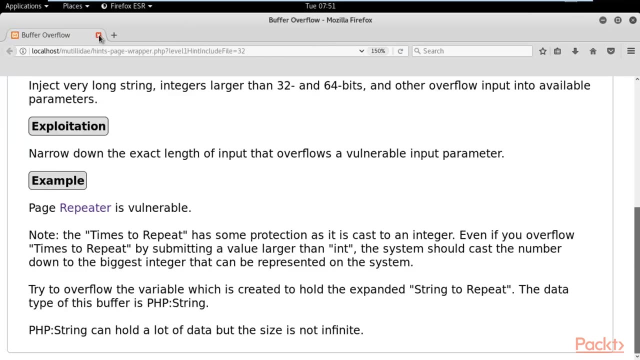 Actual web application should have limitation in the web pages, right? You cannot put more data than integer limit. And if you are able to insert more data than the integer limit, obviously this is a case of buffer overflow. All right, Now let me show you how it works. 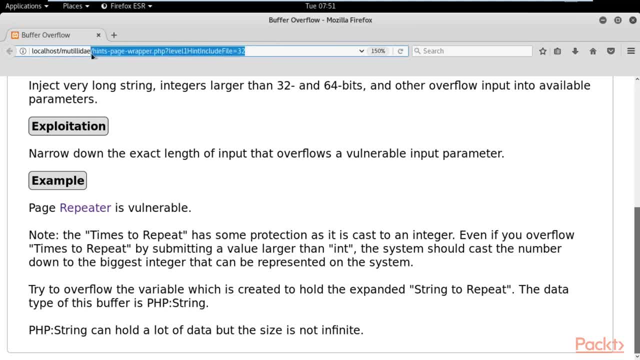 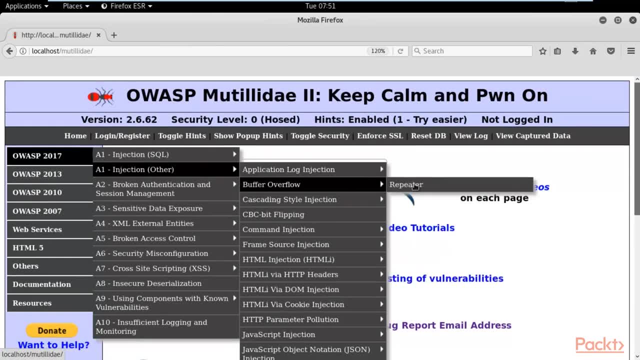 So let me go back to the Matilda local or slash Matilda hit enter And here you need to select two down: 17 other buffer, overflow and repeater. So here you can see it is asking that string to repeat, So you need to provide the string here. 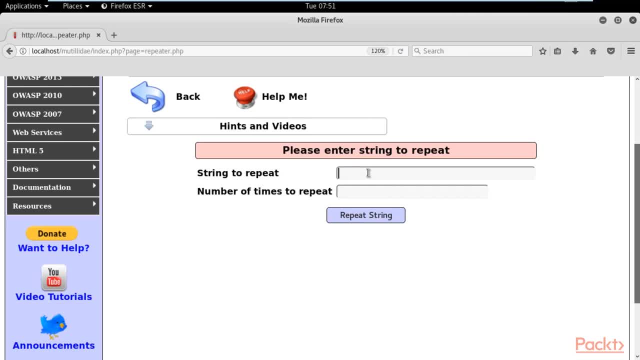 String means a kind of word, For example string. For example, my string is hello, All right, And number of times to repeat. so I can repeat the string millions of times or billions of time. if this web application is vulnerable to buffer overflow attack, for example, let 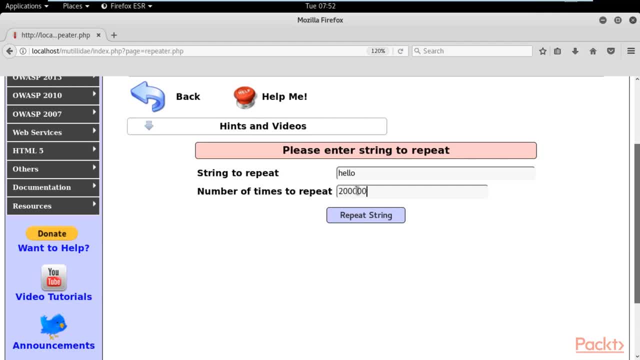 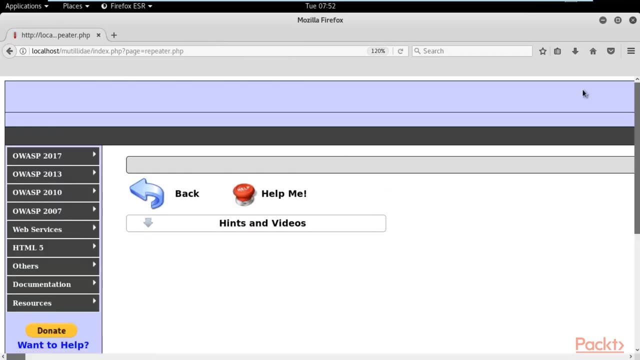 me try with 20 lakh times, because this is about the integer limit or any other limits, right? So you can click on repeat string And you can see that it is repeating And you can see here that web application has been crashed completely, right. 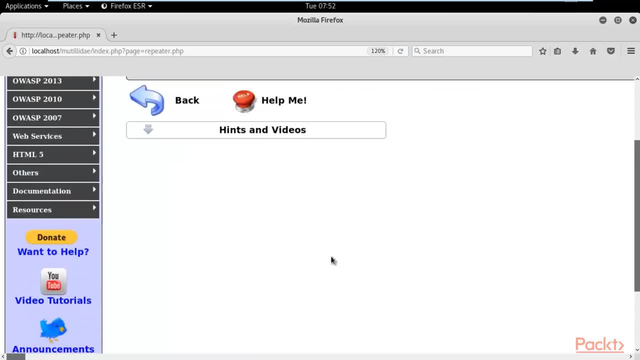 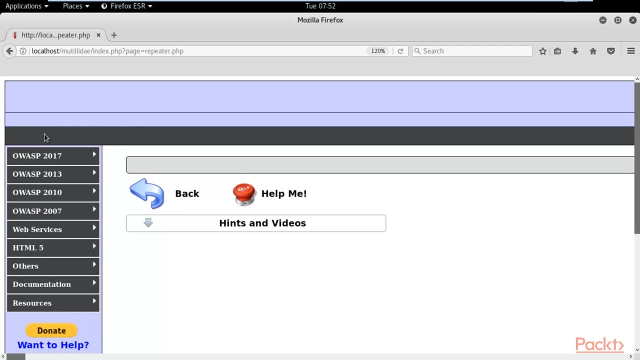 You can see here. I'm not able to see any options available here. I'm not able to do anything on this web application. So this can happen if buffer overflow is available in the web application. I have repeated that string 20 lakh times, right. 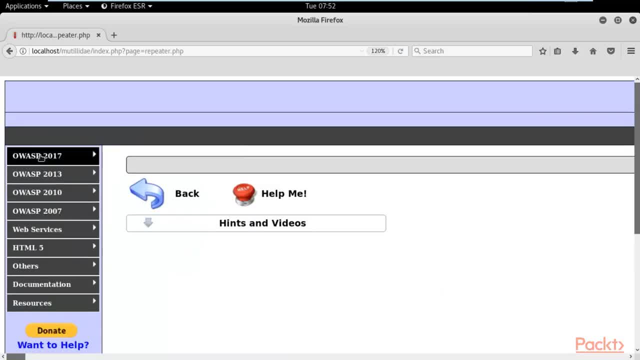 And you can see here that I'm not able to open any option which is available in the web application right. You cannot see any button available In the handset In the head part right. It means the web application has been crashed completely. 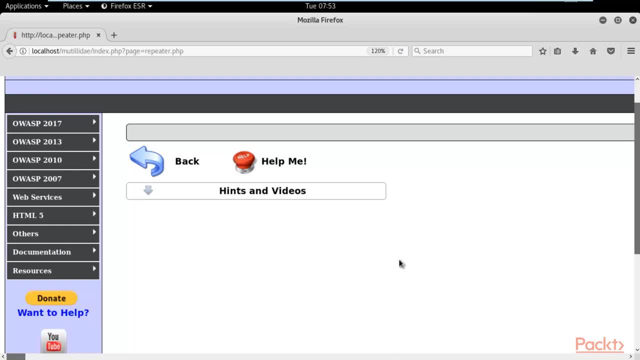 All right. So this can happen if user tries to insert more data than the space allocated. All right, this is called buffer overflow attack on a web application, And we have successfully attacked on a web application and web application is crashed now completely. All right. 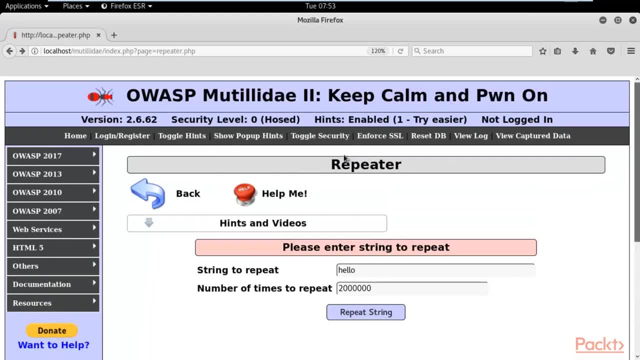 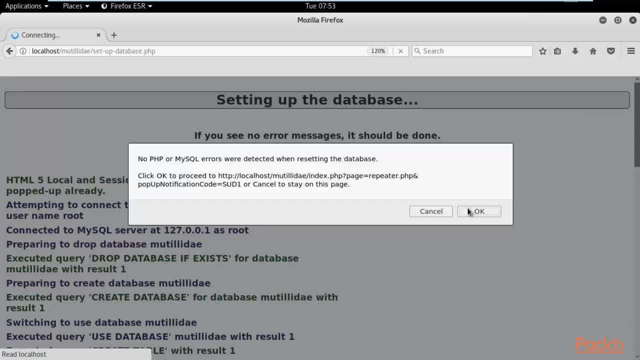 Now let me come back. And yeah, now it is fine, But at that time The web application was crashed and that was a problem because of buffer overflow attack. Now you can click on reset DB to reset your database, All right. 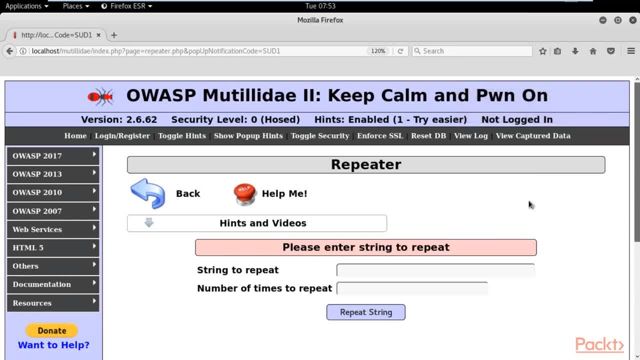 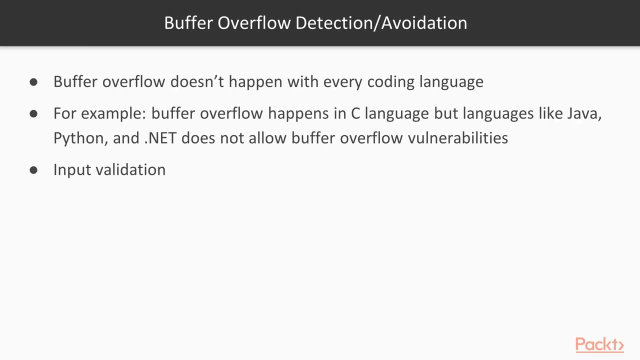 So you have learned that what is buffer overflow attack and how it works, how you can perform a practical on buffer overflow inside an application and how you can crash the complete web application by using buffer overflow vulnerability. Now the question comes here, And how you can detect or avoid this kind of vulnerability. 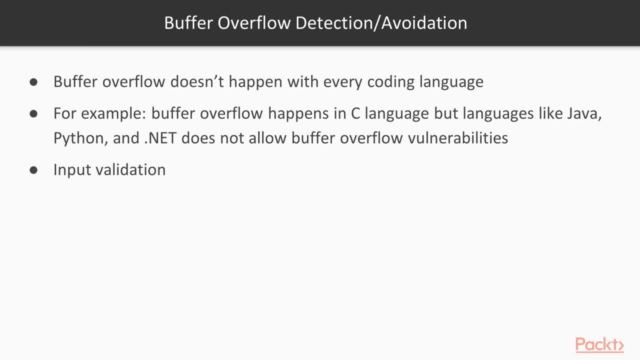 What are the best practices to avoid buffer overflow? So buffer overflow doesn't happen with every coding language. Absolutely correct, Because not each and every programming language is vulnerable to buffer overflow. Some programming languages are vulnerable and some are not. For example, buffer overflow happens in C language. 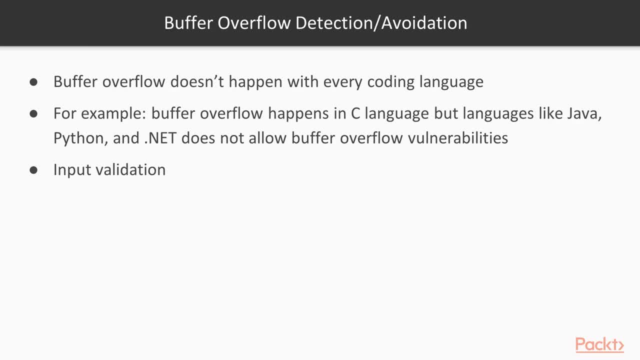 Absolutely correct. It happens in C language, But languages like Java, Python and dotnet doesn't allow this kind of vulnerability. So these kind of programming languages are secure for buffer overflow techniques. Input validation. Input validation is really important term because whatever user is inputting in that